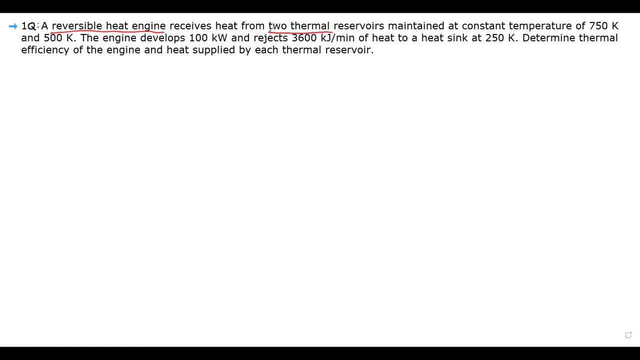 engine receives heat from two thermal reservoirs maintained at constant temperature of 7 450 Kelvin and 500 Kelvin. The engine develops 100 kilowatts, which is also called work done. rejects 3600 kilojoules per minute of heat to a heat sink at 250 Kelvin. So determine: 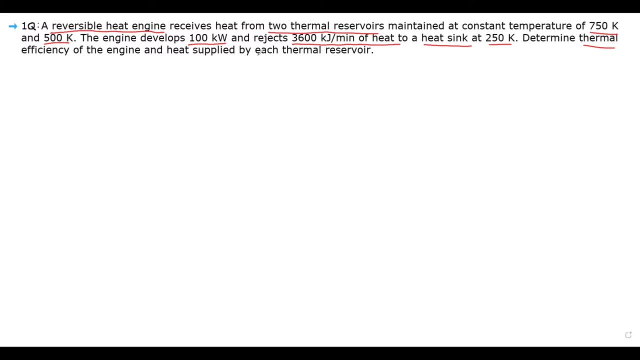 thermal efficiency of the engine and heat supplied by each thermal reservoir. So we have two thermal reservoirs here. Okay, Coming to the, let me draw the figure, then you will understand very clearly. So here we have reversible heat engine and two thermal reservoirs and one sink Clear. So 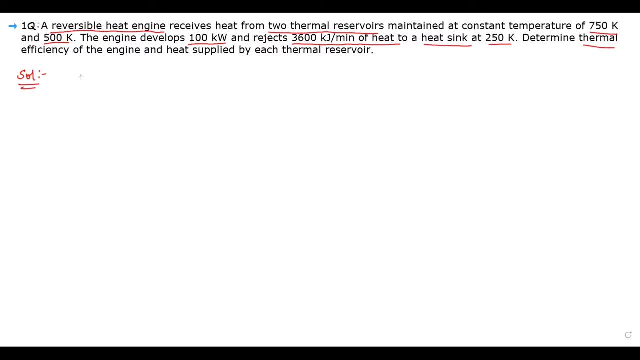 we need to have a clear idea about the figure. So let me draw the figure here, Let me choose here. This is one thermal reservoir and another thermal reservoir here And we have the sink also right, So somewhere you can draw the sink here. So this is called the sink, And 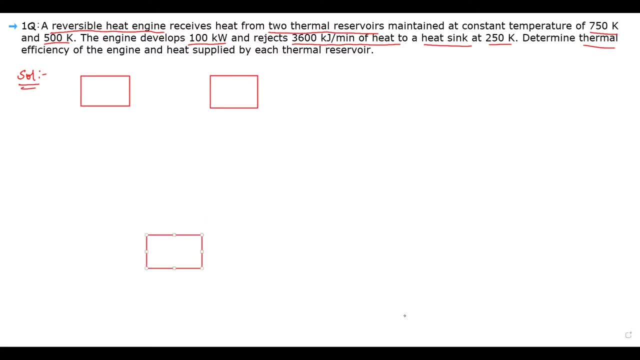 in between, we have the reversible heat engine right, So let me draw here. This is the reversible heat engine. Clear, And now here we are. there is a heat transfer which is taking place from two reservoirs to the engine. 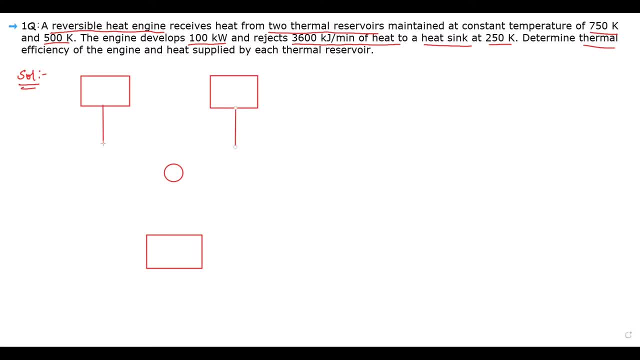 So this is the heat transfer. So this is the heat transfer. So this is the heat transfer. There is an economy. There is a diskut báse dans ceci. Now, look at to this figure, Now, here, let us consider now this is thermal reservoir. 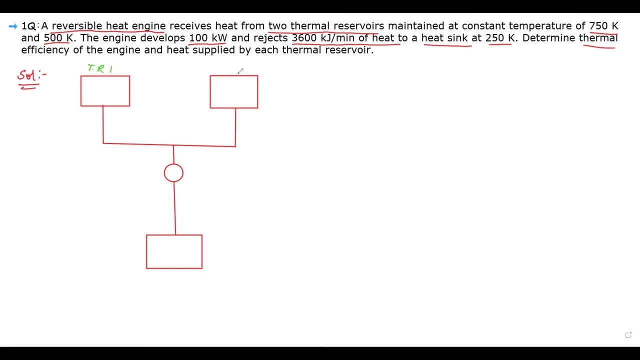 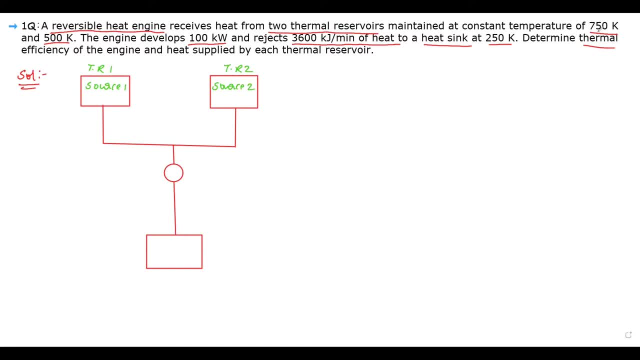 temperature is given, that is called the thermal reservoir. one temperature is 750 kelvin, so here it is 750 kelvin, and here source 2, which is 500 kelvin, and now which is called the engine, this is called engine, right, and this this is called reversible heat engine and which develops. 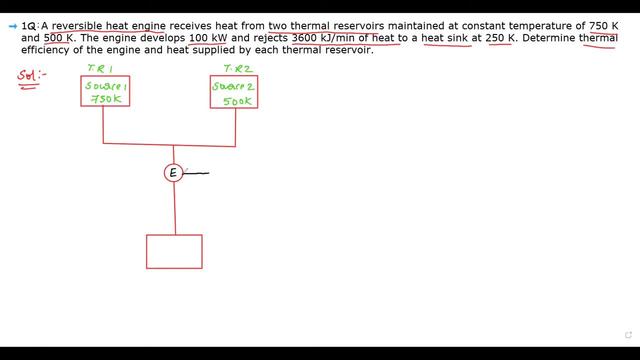 which develops work output that is called work done, work output, which is equal to 100 kilowatts. 100 kilowatts, so i will convert into kilojoules per minute. so 100 kilowatts, which is also equal to 100 kilojoules per second, so 100 into 60, then we will get in terms of: 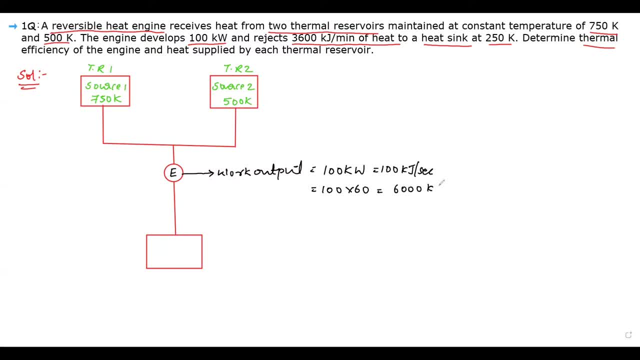 6000, so kilojoules per minutes, right, and then after. here, the heat which is supplied to the engine from source 1 is q1 and source 2 is q2, then total heat is supplied to the heat engine is q1 plus q2, right, and then here, after this work, output. 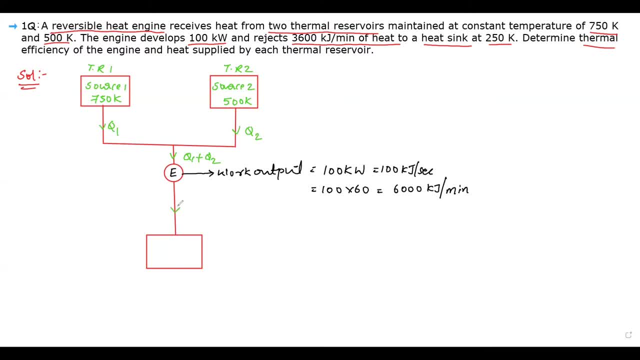 the engine will develop, produce, release or supply the or reject the heat to the heat sink, which is equal to how much heat rejection is 3600 kilojoules per minutes. then here it is 3600 kilojoules per minute and this is called heat rejection. this is called heat. 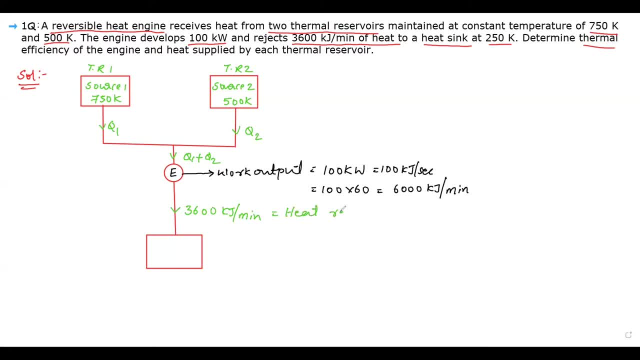 rejection. and here is q1 plus q2, which is called heat supplied to the engine, right heat supply, and here which is called boiling plate. so this is for injuries, and it is called question 8, which is quickly replaced and this time it will get different per unit panelized product and after which we put 4 Túmeros, there will be total olmasso in the engine, so it will be water Commercial Nit molds and therefore these are both additional in-ship cutting groups which are lying fromhere and now. these are all favourites for reverse engineering. are there we have to use a sink, is we can suggest and support them between the three points? so, or do we want somethird of twice to system to work? condition of these. 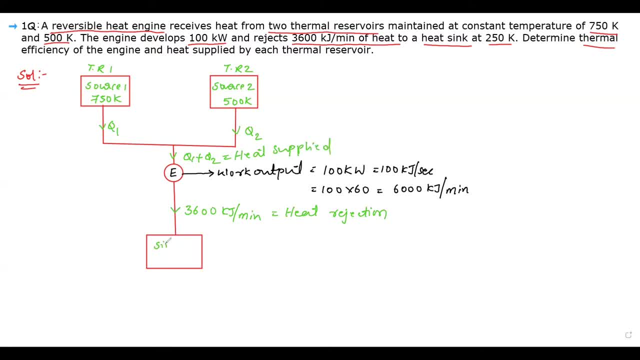 applied and here which is called the sink and where the temperature is given 250 kelvin. right now, look at what we need to find here. we need to find the first bit. let us consider in terms of bits. first bit is thermal efficiency- thermal efficiency. and second bit, we need to calculate. 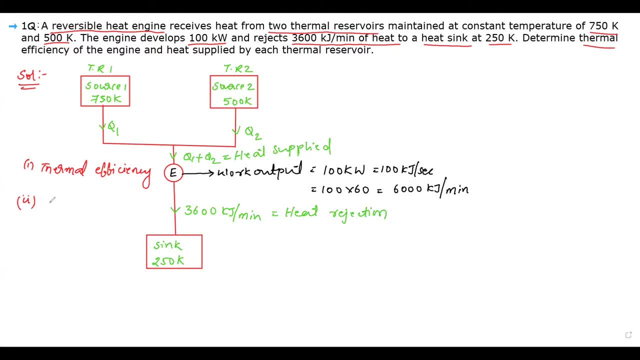 or we need to determine heat supplied by each thermal reservoir. heat supplied by each thermal reservoir right now. here let us consider first bit now, that is, thermal efficiency of the heat engine, right, thermal efficiency of the heat engine, right. so thermal efficiency, which is equal to the ratio of- we know that- the ratio of work done. 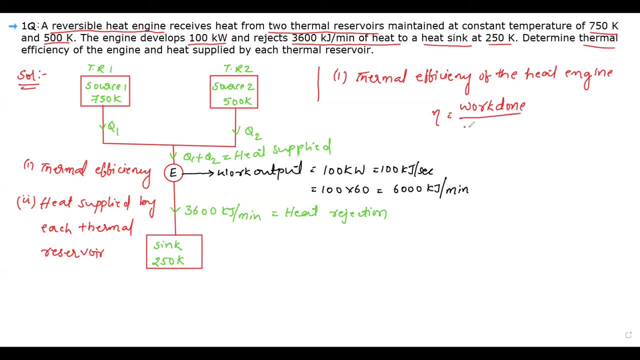 to the heat supplied. heat supplied, clear, but look at here the work done already. we know that is a 6000 kilojoules per minute. but heat supplied we need to calculate because which is not there, heat supplied, which is equal to q1 plus q2. 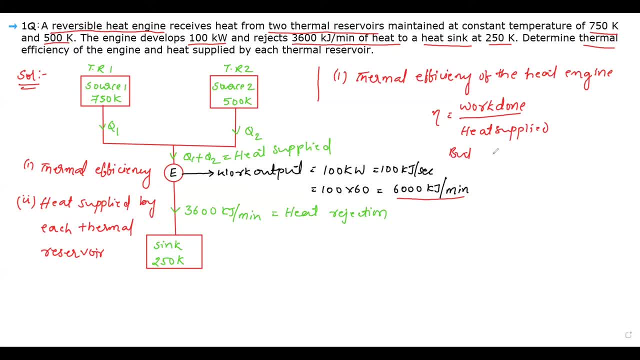 but we know here, but we know that, we know that very simple, we know, we know that work done which is equal to work done, which is equal to heat supplied. in the shortcut I'm reading heat supplied minus heat rejection. right now, here we need to calculate heat supplied. so 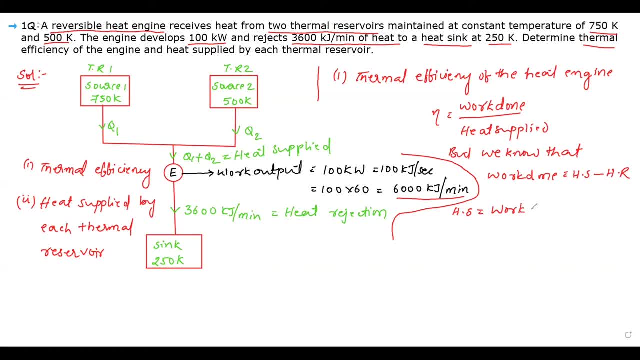 he surprised that, which is equal to what some of the equation work done plus he projection. so how much? how much is betel here, which is 36,000, and players he Salvartis, they'll heat supply, which is equal to 9600 kilojoules per minute. kilojoules per minute. So we know the work done and we know. 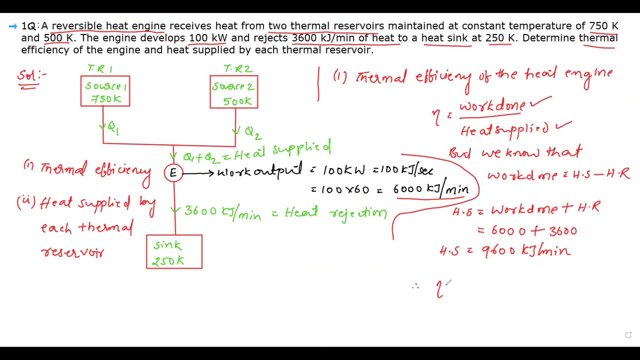 the heat supplied, then we can get the. therefore, thermal efficiency of the heat engine is work done is 6000 divided by heat supplied, which is equal to 9600, and it will give the approximately. you know, this 2020 will gets cancelled right: 60 divided by 96.. So 0.625, 625. or we can say: 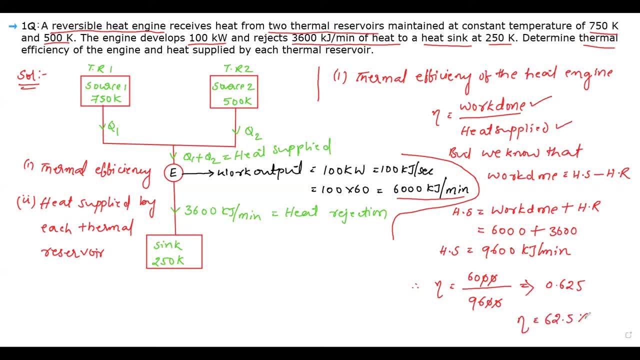 which is equal to 62.5 percentage. So the efficiency of the heat engine is how much 62.5 percentage? So first bit is over, right next we need to go for the second bit. So what I? what I need to do now? I need to erase, because I do not have space, So I am erasing. 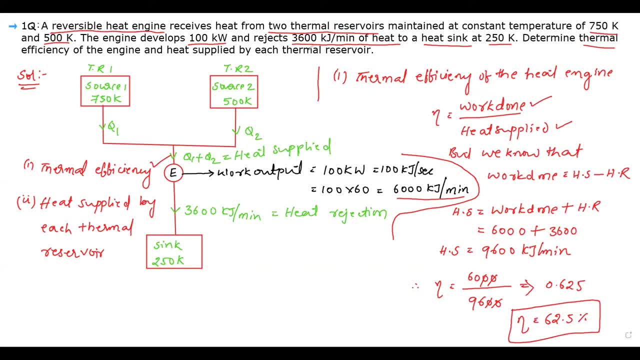 now this first bit that enter calculation part. So just give me a minute. very easy. you need to know the basic equations right, and basic concepts of first class thermodynamics right and applications of first class thermodynamics. I think very easily you can solve the problems. 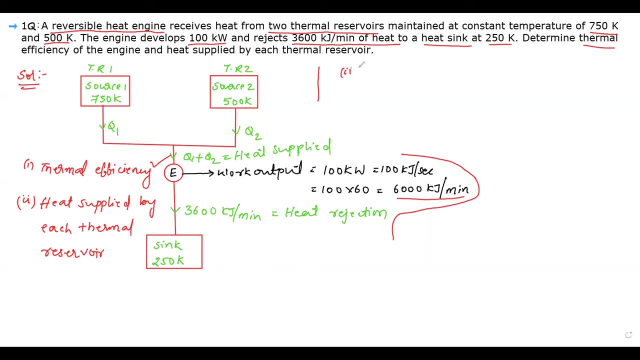 Now next second bit. Second bit: what we need to calculate here, what is the heat supplied by each thermal reservoir, Heat supplied by each thermal reservoir. So we have how many thermal reservoirs, How many thermal reservoirs, How many thermal reservoirs. 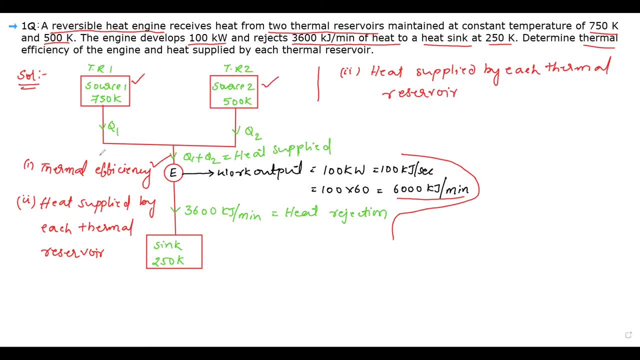 We have two, that is, source 1 and source 2, here. From source 1, let us consider Q1 and from source 2 it is Q2.. So we know that Q1 plus Q2, which is equal to total heat supplied, is how much just now we have calculated, which was equal to 9600 right kilojoules per minute. 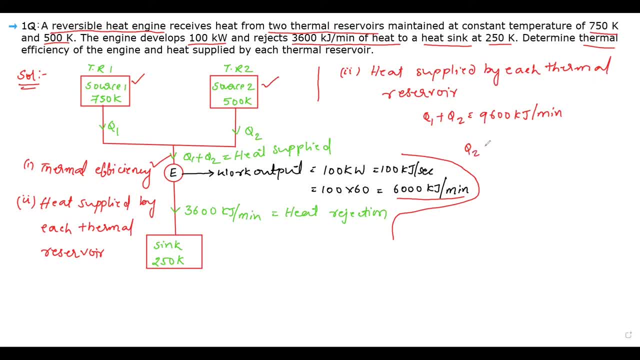 So where what I will do now? then Q2, which is equal to how much 9600 minus Q1.. Q2 is equal to how much 9600 minus Q2.. So this is equal to how much 9600 minus Q2.. So this is equal. 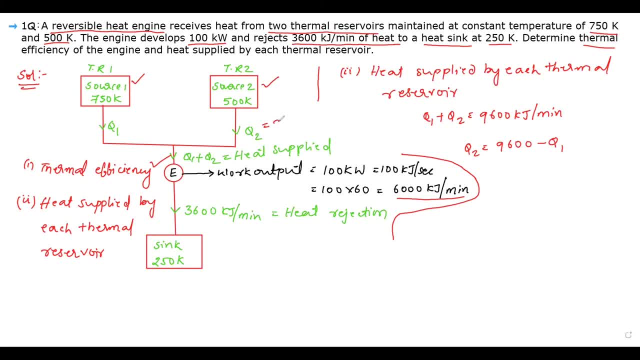 to how much 9600 minus Q1.. So here, right, Q2, which is equal to 9600 minus Q1.. So, according to classiest theorem, according to: or I will write here, as the engine is reversible, right, Right, Right. 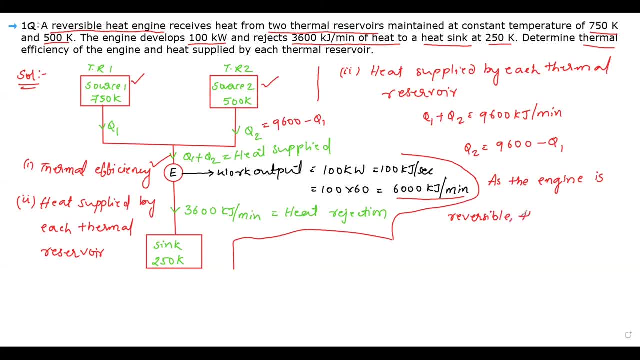 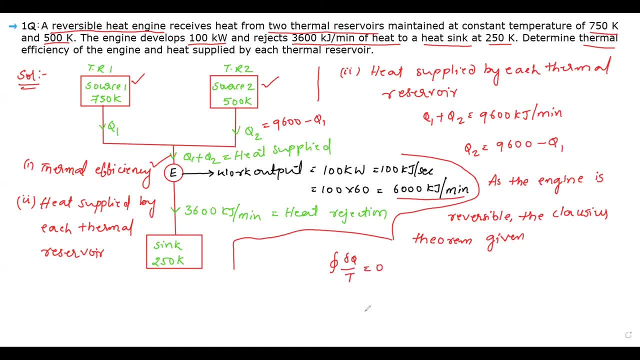 right, which is equal to what Zero understand. Now, here, ratio of heat should be treated in wheat. it is the ratio of heat to the temperature, right? So let us consider first the source, one where heat supplied is Q1 divided by where the temperature is 750, right And plus, because here 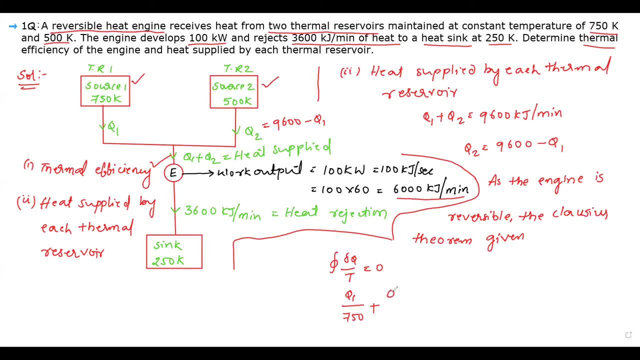 it is Q1 plus Q2, that is called heat supplied, right. Then it is Q2 by 500, clear And minus, because heat rejection, heat rejection, which is equal to how much? 3600, right, So 3600 divided. 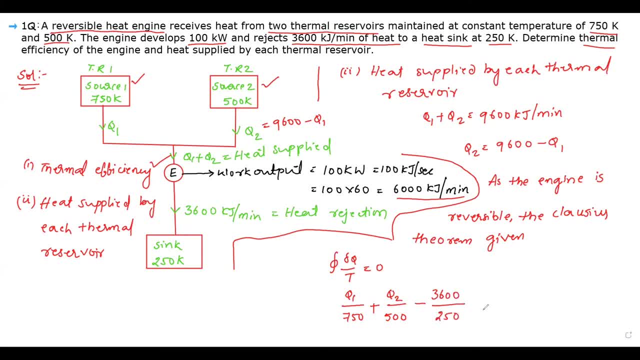 by where the temperature is how much? 250, which is equal to what Zero according to Eboi equation, right? So here, according to Eboi equation, Q1 is Q1 divided by 750 plus Q2 is equal to how much? 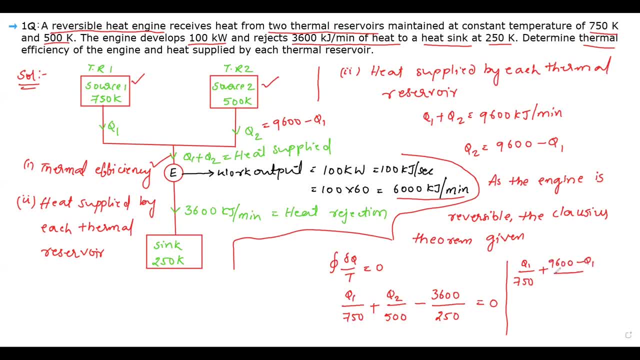 9600 minus Q1 divided by 500.. 500 minus 3600 divided by 250, which is equal to what? Zero right From this equation? look at here in this only Q1, we need to. we can get the Q1 answer right. So if you simplify this, you. 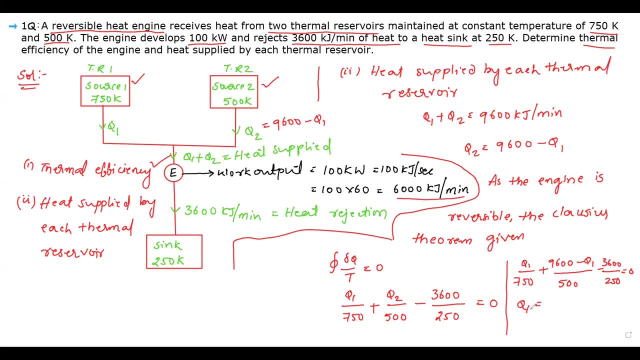 will get Q1, which is equal to just a minute. let me calculate Q1, which is. we can take so 750, 500, Q1, which is equal to 7200 kilojoules per minute. kilojoules per minute Next, what we need to.